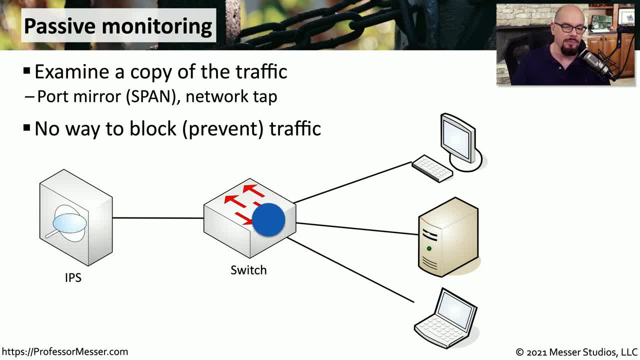 And a copy of that traffic is sent to the IPS. during that process The IPS then examines that copy of the traffic flow to see if there's any known attacks inside of that traffic. If there is, usually an alert or a message is displayed so that the system administrator can then 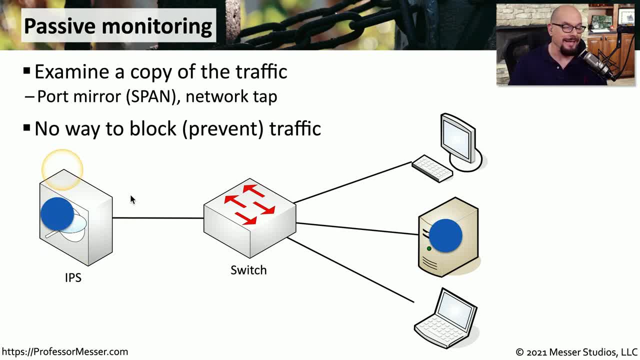 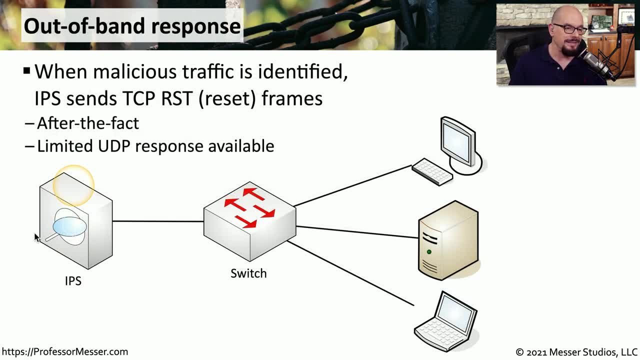 decide what to do next. Since this IPS is not in line with the actual traffic flows, there's no way for the IPS to block that in real time. If the IPS is in one of these passive modes, then they're not in line with the actual traffic flows. 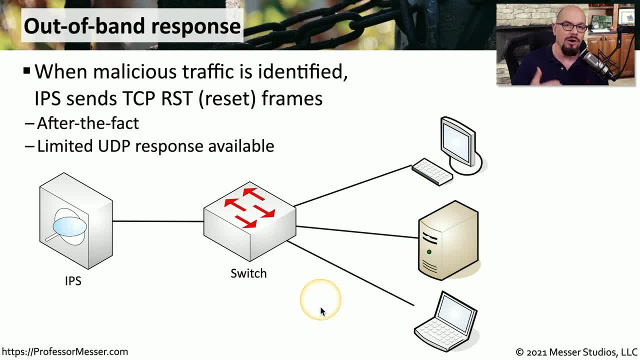 and cannot block that traffic in real time. However, there are some response methods that would allow the IPS to limit the amount of traffic that might be sent or received from a device. once that particular malicious traffic is identified, We do, We set through an out-of-band response. 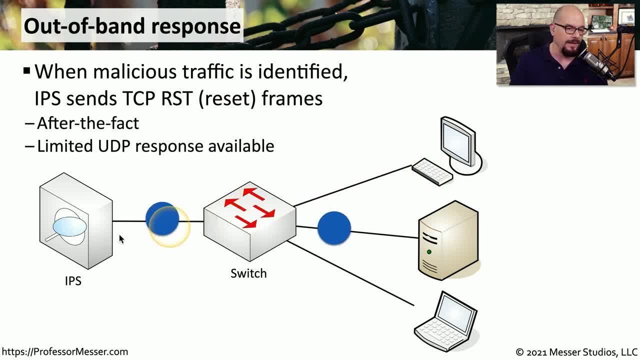 We have traffic that's going between systems, A copy of that traffic is sent to the IPS. If the IPS identifies malicious traffic within those flows, it can send a TCP reset frame to these devices, effectively disabling that particular traffic flow. This doesn't stop the original packet. 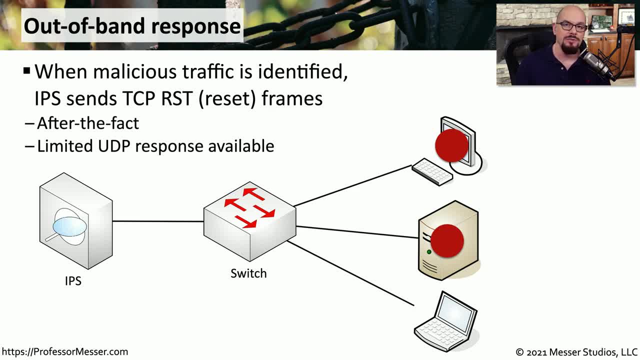 from getting through this conversation, but it would prevent any subsequent information being sent over that same flow. This reset functionality is part of the TCP TCP protocol. If the traffic flow was one that was UDP-based, the IPS would not have a reset feature. 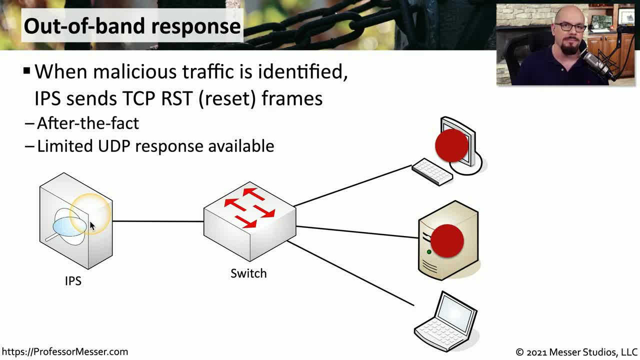 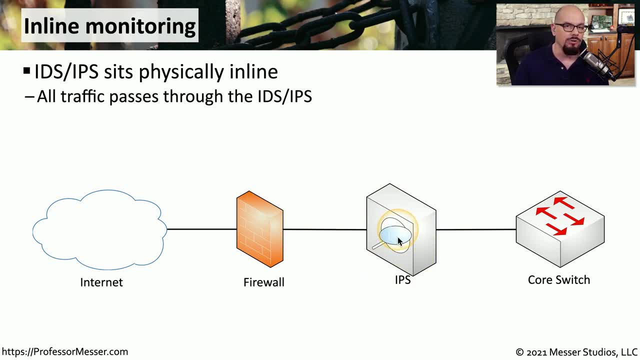 available to be able to disconnect that particular flow. A much more common implementation for an IPS is to have the IPS in line on the network, evaluating all traffic that's sent through it. Traffic is sent into the network and received by the IPS. The IPS then examines the traffic. 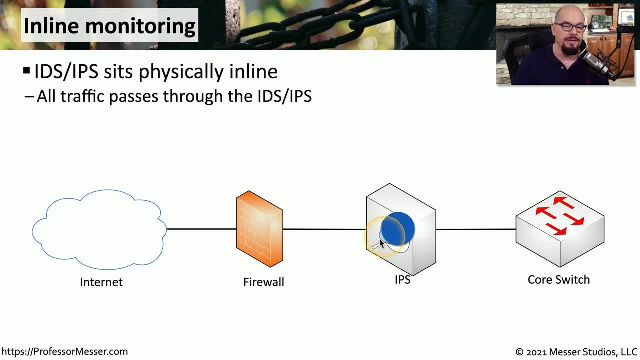 makes sure that nothing inside that traffic might be malicious, and if everything looks OK, it sends it online. OK, And if it's not, then the IPS is in the way. Because the IPS is in band, it's able to block the traffic. 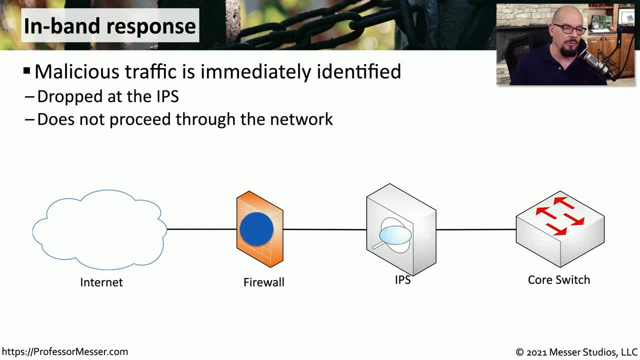 in real time and prevent any of the malicious traffic from getting inside the network. So the same traffic flow would occur and as that traffic hits the IPS, the IPS would recognize that there's some type of attack inside of that packet. It would then drop that packet, prevent any additional traffic.